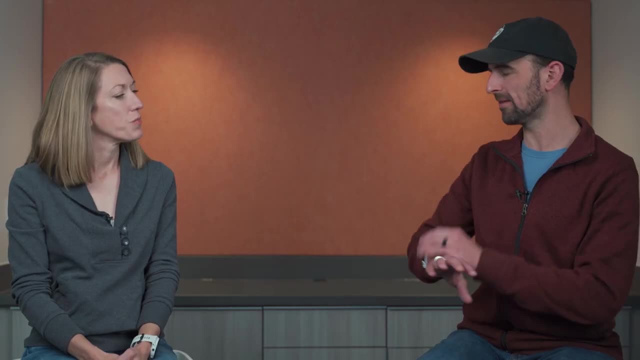 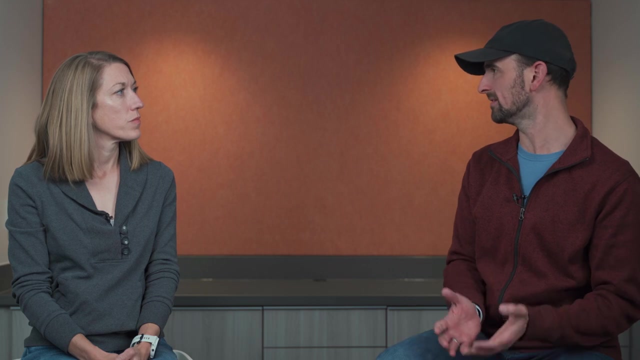 like how you're recovering. How would somebody who has a watch that's compatible with HRV and HRV and has HRV status on it? what steps do they need to take to be able to do that? What steps do they need to take to start getting metrics and getting their HRV metrics? 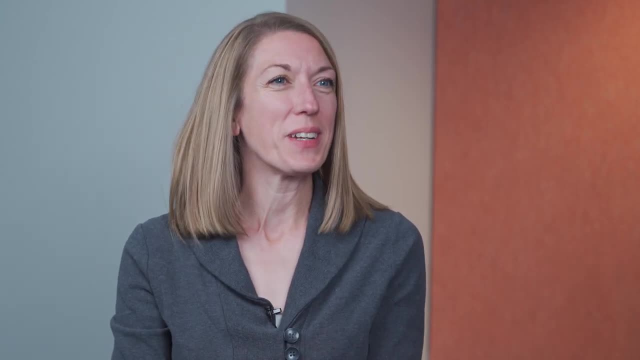 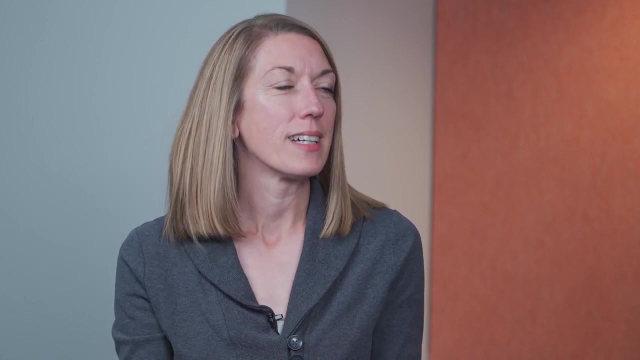 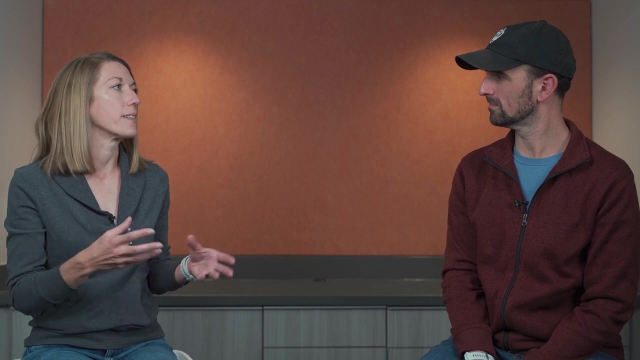 It's really easy. The beauty of the HRV status is that there's really no user input required. The most important thing is that you just wear the watch to sleep. We try to kind of build up as much information as we can about your overnight to try and remove like anomalies or spikes or 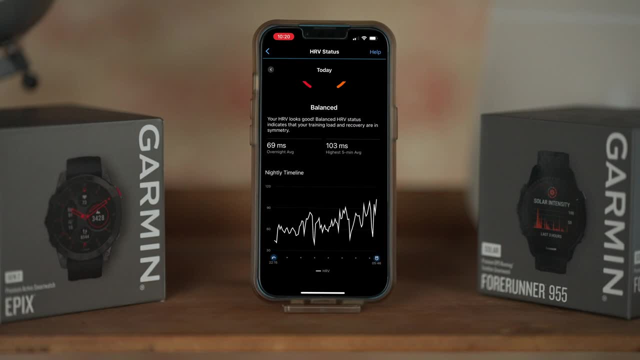 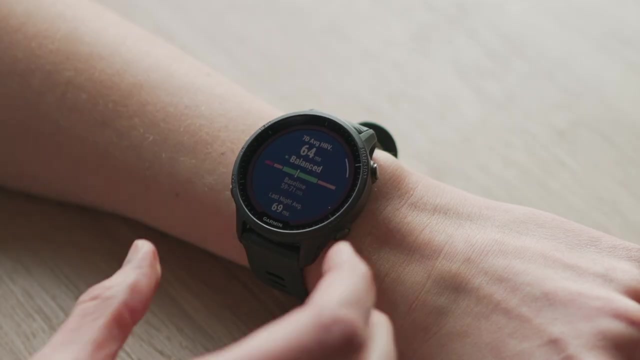 differences that might not be. Once we've gotten a week's worth of those overnight HRV values, we'll provide a seven-day average HRV And then over about a three-week period, once you've been wearing the watch to sleep, we can build up enough information about you, enough history to understand what your. 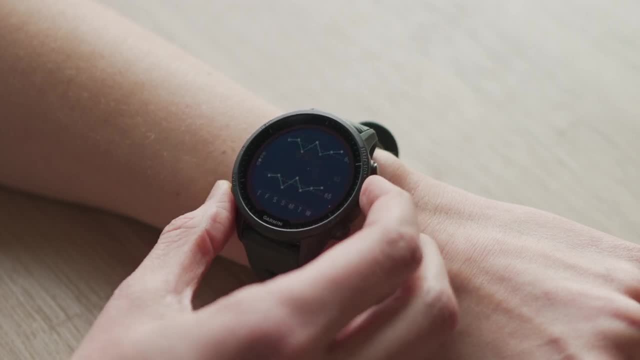 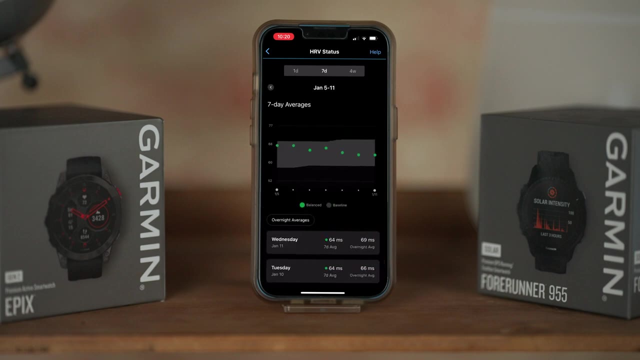 personal baseline range is. So what's a normal range of HRV values for you? And then we use that to. we compare your seven-day average So you can look at your personal baseline range if you're going to be wearing a watch. 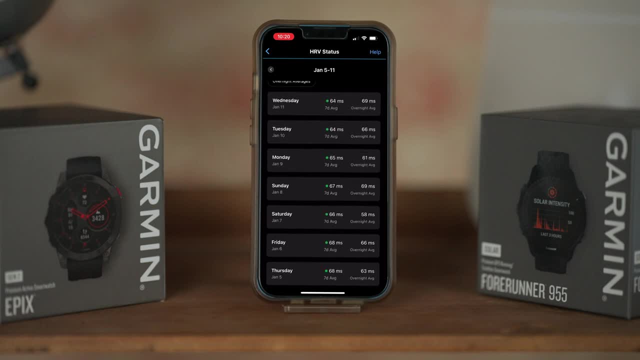 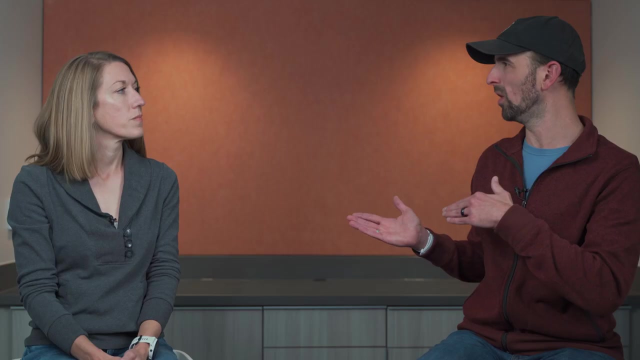 So you know, you can use that to tell you your personal baseline range, to tell you whether your HRV is currently in balance, which is a good sign that your body is in homeostasis and that you're, you know, adequately recovering from, you know, any training load that you've put on your body. 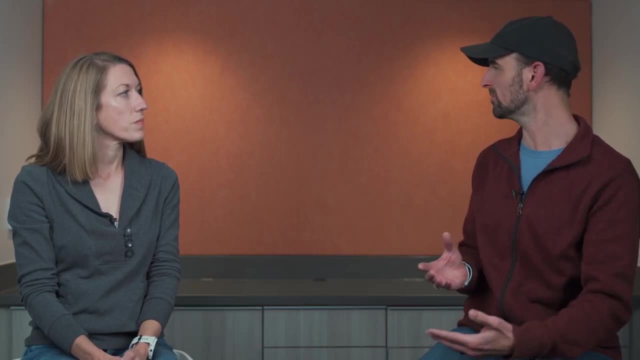 stress that you've put on your body. If somebody is unbalanced on either side, what is? is there a general idea that any customer could be able to kind of determine based on that? What about your personal baseline range? What does that look like? 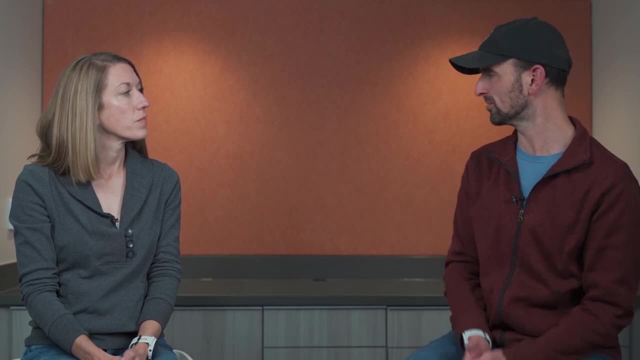 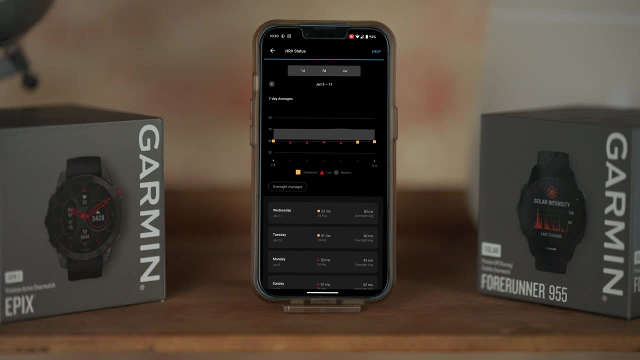 How much training have you been doing recently? Have you ramped up the amount of training or have you been doing more intense training than usual? Maybe you know if you see that you're in the unbalanced and you're staying in the unbalanced. 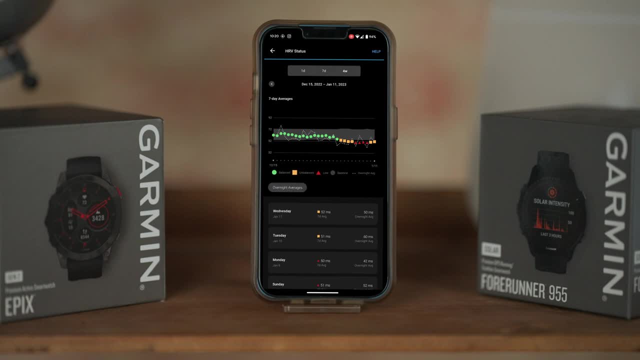 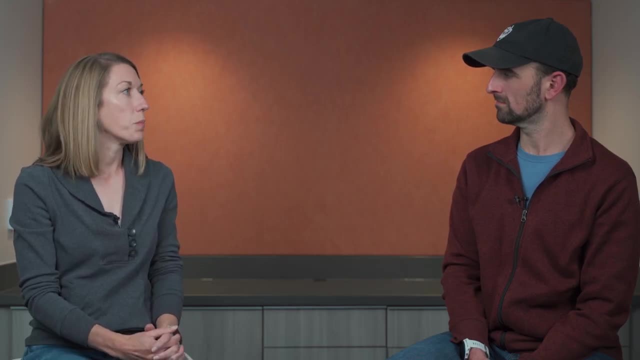 then you know that might be a sign okay, maybe I need to back off on my training a bit, get a little bit more rest. Could be other factors as well, You know, just looking at like sleep, sleep habits.